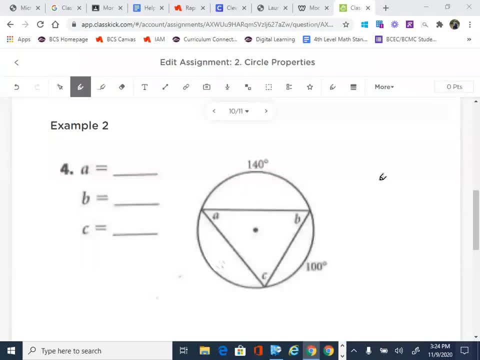 All right, we're going to be looking at circle properties and, in this case, we're going to be focusing on the arcs and their inscribed angles. All right, so we're going to find A, B and C. It does not matter where we start in this one, so let's go ahead and try A first. Okay, so what? 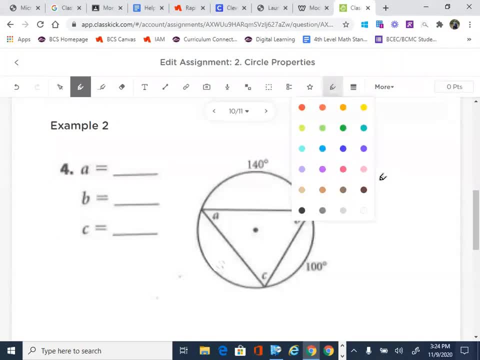 you'll notice about A is, or should notice about A is that it is a inscribed angle and it is part of this beautiful triangle that is right there inside that circle. So look at A right here. I'm going to go ahead and shade it and one thing I notice is that it completely grabs this arc right. 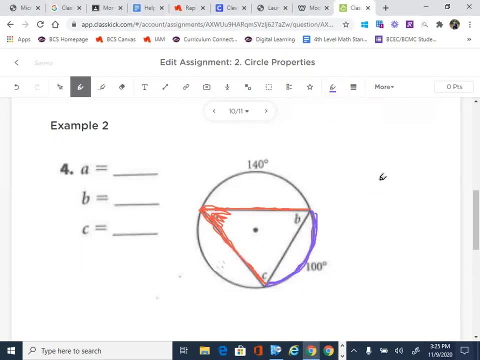 here. I kind of like to call of it a snow cone. You got the cone and you got a little snowball right over the top of it, Okay, so anyways, it comes in and it grabs that arc and we know is an inscribed 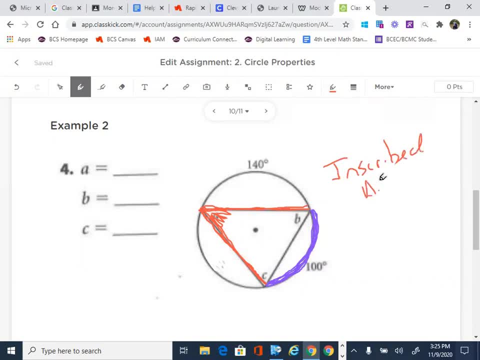 angle Is one half of the arc that it intercepts. So in this case, in order to find A right here, we are simply just going to take one half of 100.. Okay, so A would be one half of 100, which is 50 degrees. 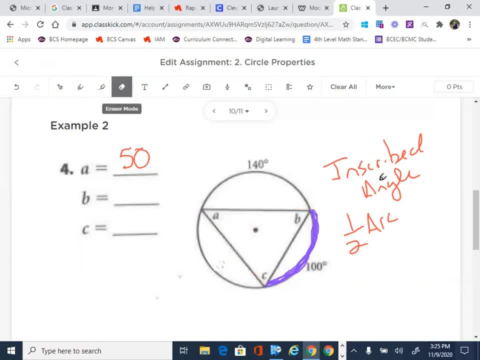 You can put that into Desmos if you need to. You couldn't make that calculation. Now we know that there's 100 degrees there, and what I look at is I say, well, what's next? What can I find next? Well, 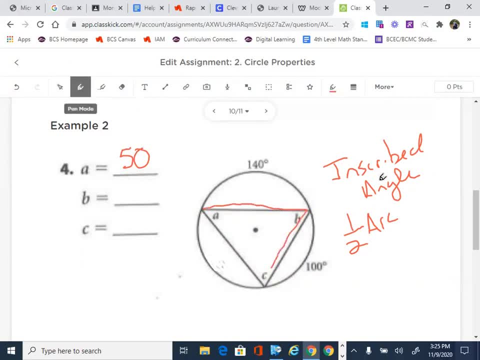 if I go to B at this point. well, check it out. I go to B, I have an arc, but there's no actual degrees there. but we can find that if we want to. So notice what's happened. I have a 100 degree arc right here and I have a 140. 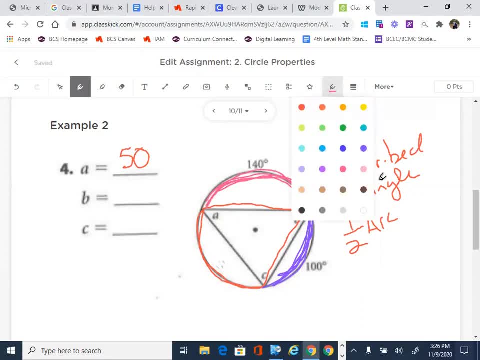 degree arc right there, and what I'm looking for is- maybe I can find this arc right here, because that is going to help us find B. How many degrees are there in a circle? There's 360 degrees, So we start with 360, and we subtract. 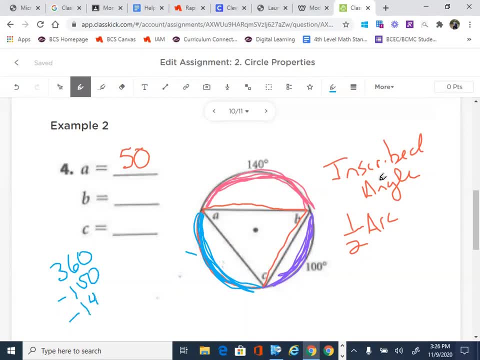 off the 100, and then we subtract off the 140.. So, in other words, we take 360, and we subtract 240, right, So we have 0,. 6 minus 4 is 2,. 3 minus 2 is 1, so that's got to be 120 degrees You may have.